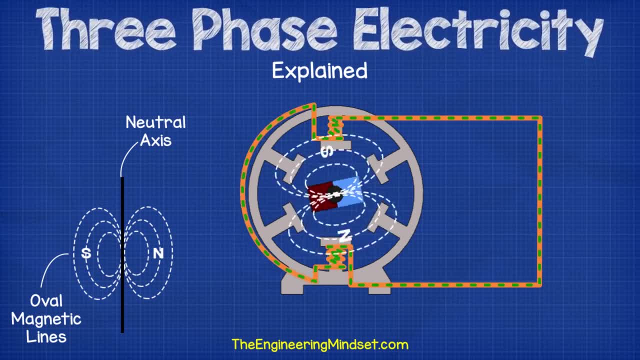 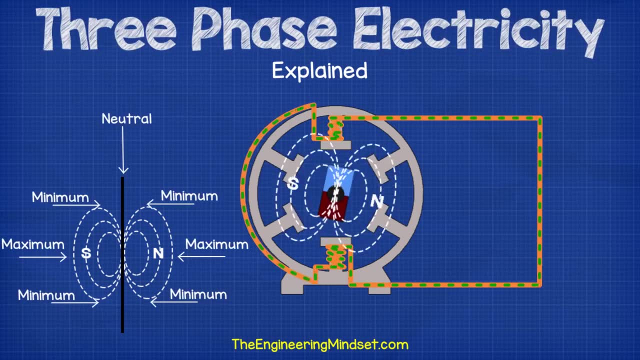 meet through the central axis of the magnet. You can think of these as one side being positive and the other side being negative, and in between these ovals the magnetic field is neutral. You can see that the intensity of the magnetic field is much higher than the magnetic field on the other side of the magnet. 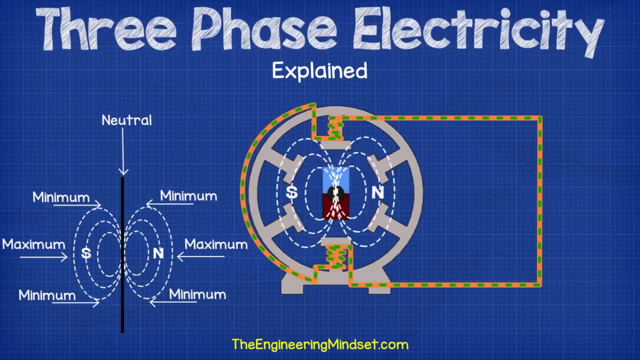 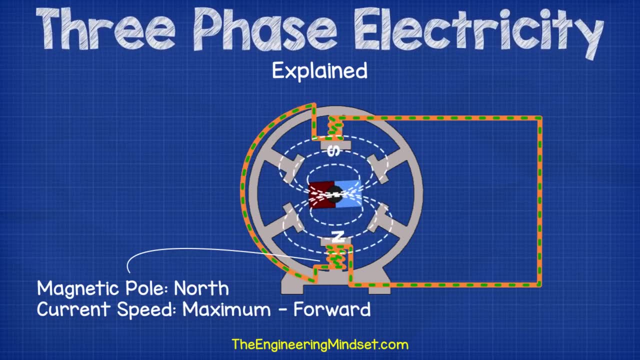 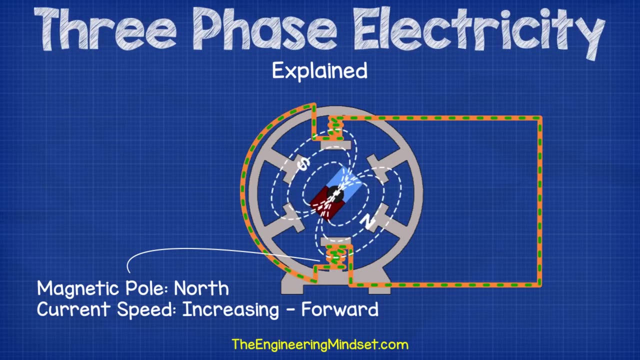 The magnetic field increases on either side until the centre, where it is at its maximum strength, and then it decreases again until it gets back to the neutral point. So as this field rotates through the coil, the coil will experience an increasing intensity of the magnetic field's positive half and during this increase the free electrons within. 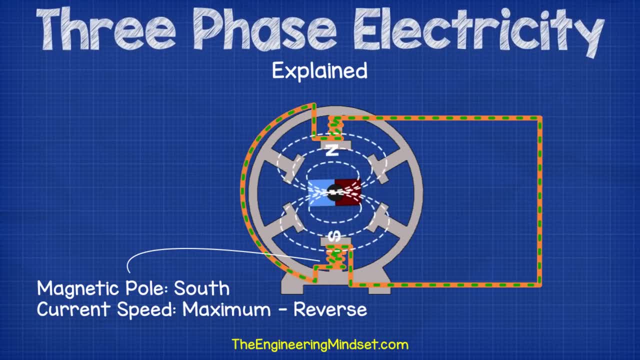 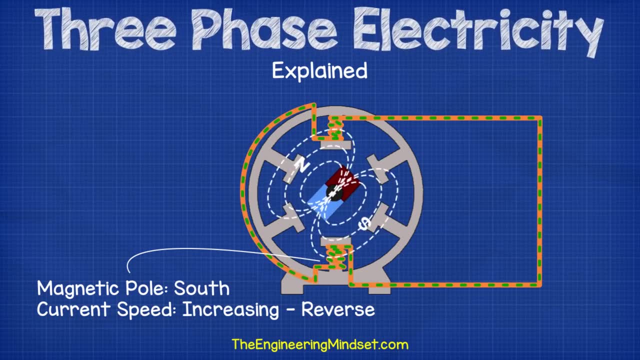 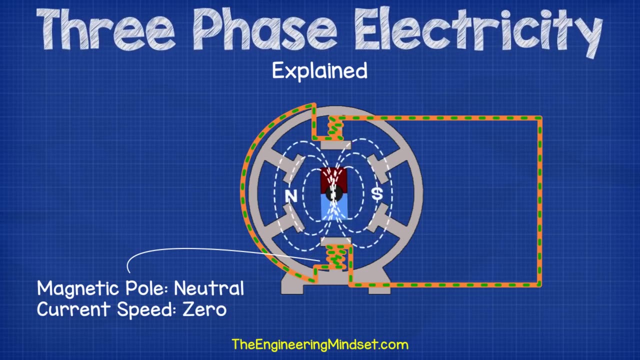 the copper coil will be pushed and begin to move faster and faster in one direction up until it reaches the maximum point of the magnetic field. As this field decreases, the flow of electrons will begin to slow all the way until it reaches the neutral point, where no electrons will flow. 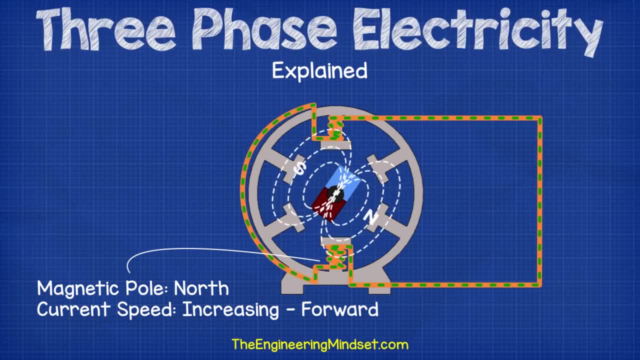 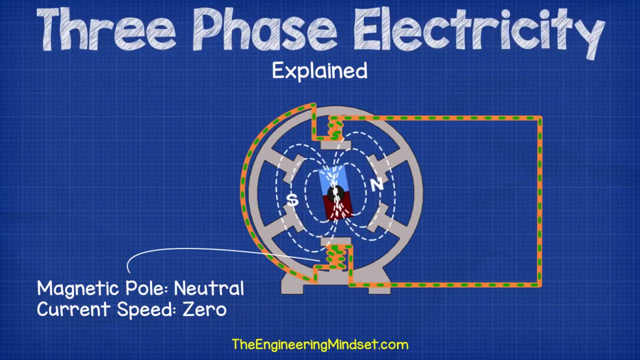 Then comes the negative side of the magnetic field, and as this passes through it's going to pull the free electrons backwards Again. the flow of electrons will flow faster and faster up until the maximum point of the magnetic field, and then it will decrease. 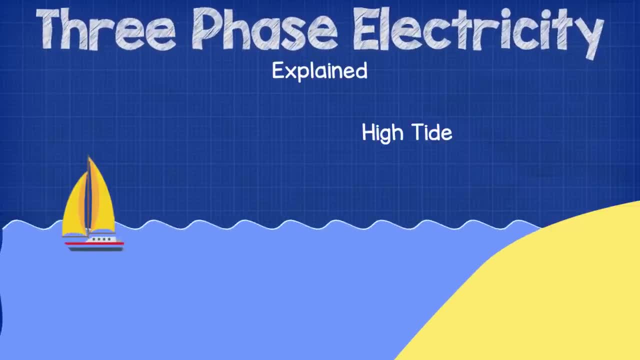 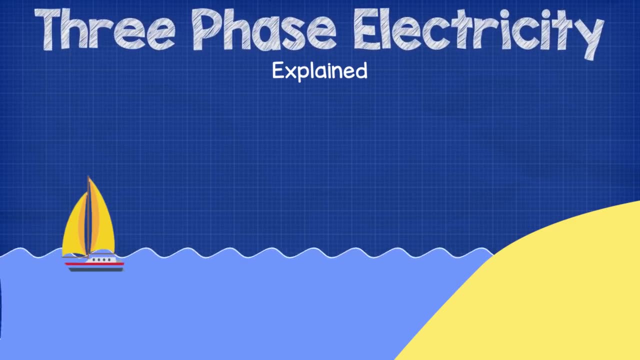 back to the neutral point. This is why AC electricity is called alternating current, because the current of electrons alternates in direction, backwards and forwards, just like the tide of the sea. If we were to plot on a graph the speed of the electrons flowing during the rotation, 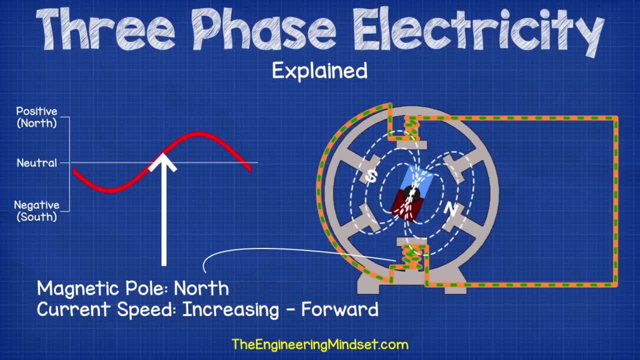 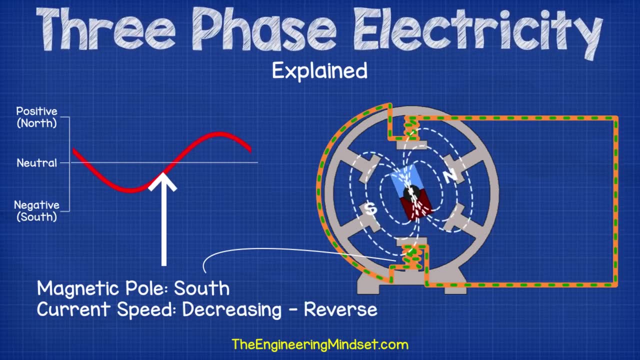 then we would get a sine wave pattern. In this sine wave you can see that the electrons are stationary at the start in the neutral zone, and then the speed increases through the positive half all the way up to the maximum, and then it begins to decrease all the way back down to the neutral, where no electrons 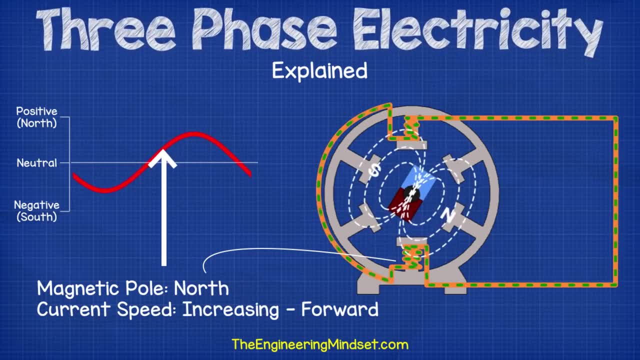 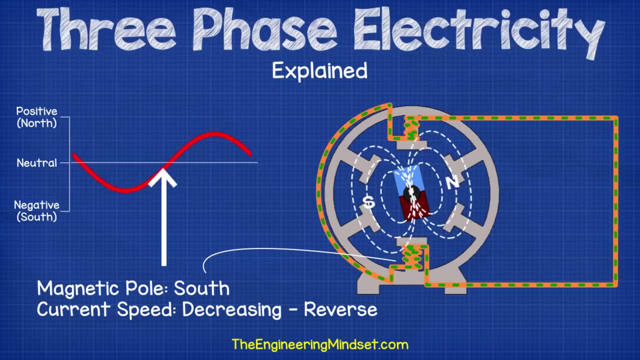 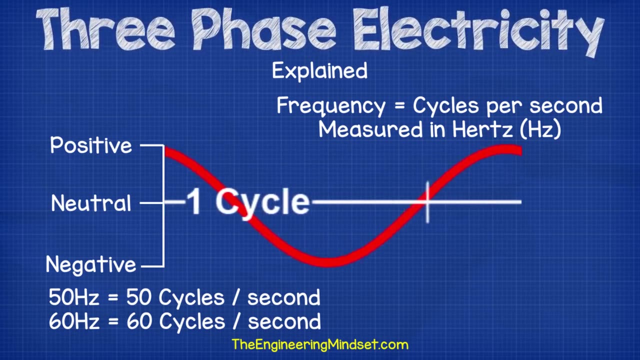 will flow again. After this comes the negative half, where the electrons will continue to flow up until the maximum point and then they begin to slow down again until the magnet has completed one full rotation, where this will then repeat. This complete rotation is known as a cycle, and the number of cycles per second is called. 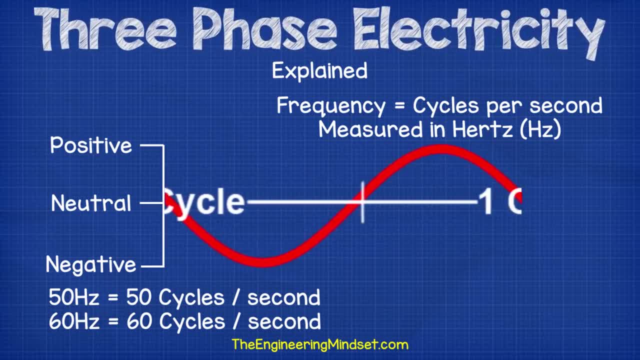 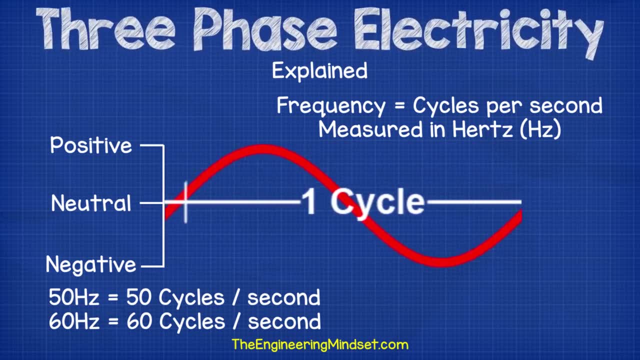 the frequency, which is measured in hertz. You've probably seen 50 hertz or 60 hertz written on your electrical goods. This means that the generator of the power station is completing a full rotation either 50 or 60 times per second. 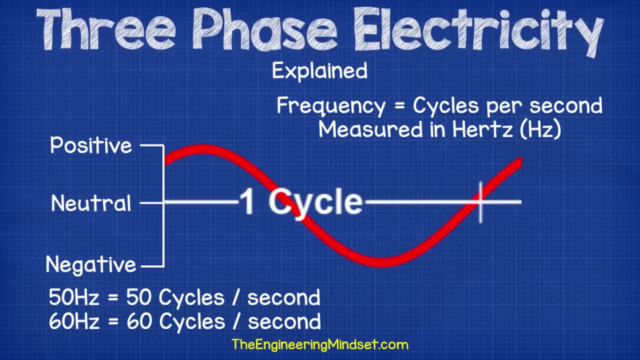 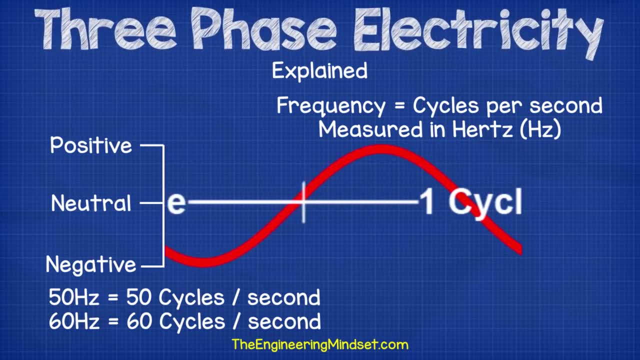 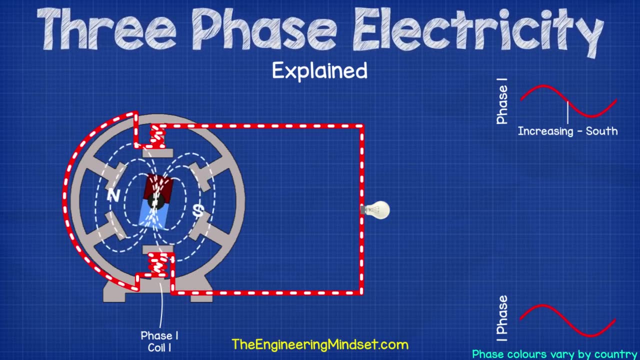 The direction of the current is therefore also changing 50 or 60 times per second. also, When it is written on electrical products, this is just telling the user what type of electricity the product should be connected to. Now, coming back to the sine wave that we saw earlier, this plot of current also represents 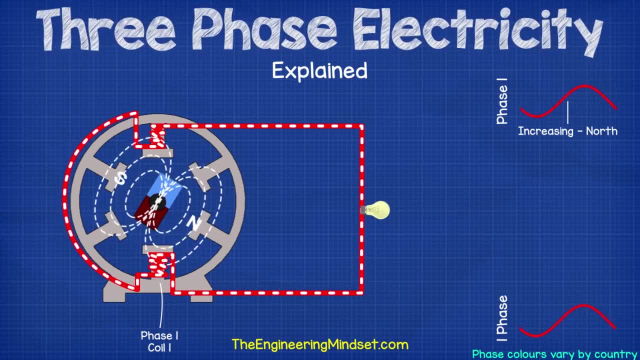 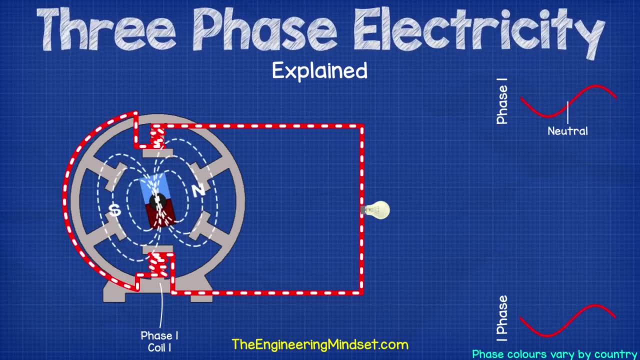 power and if we connect a lamp into the circuit, we'll see that it will increase in brightness all the way to the peak, that maximum point. then it decreases in brightness all the way down. This is the point where the lamp is actually off because no current is flowing. 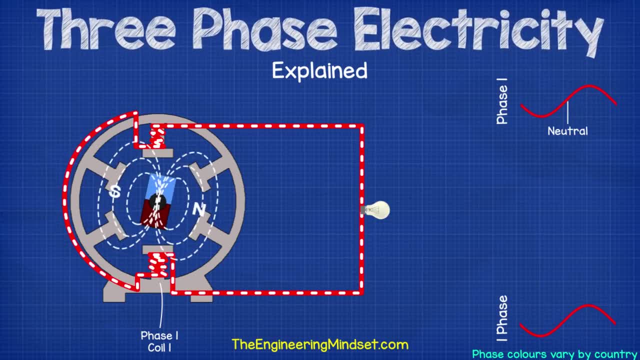 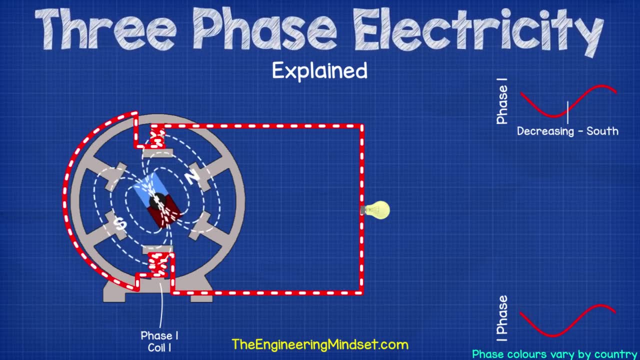 But then it will increase in brightness again as the negative half of the cycle comes through and the electrons start to flow back through in the opposite direction, until again it reaches the neutral point. So at these points in the cycle the lamp is not producing any light, and at these points, 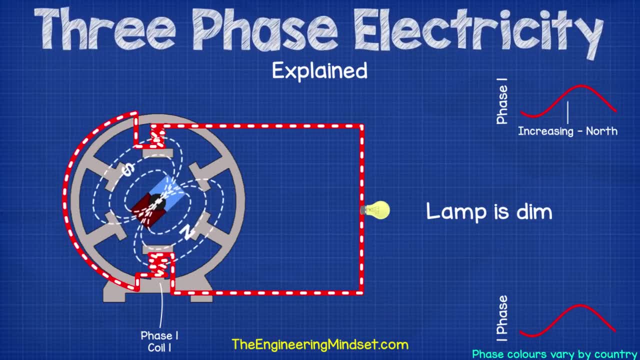 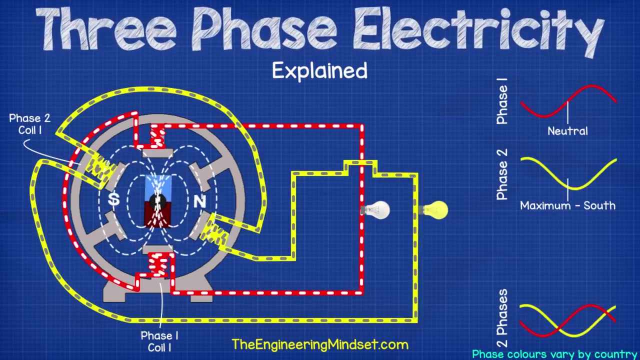 in the cycle. the lamp is not very bright, so it's not of much use. So if you're working in a room and this lighting is flickering like this, it's going to get really annoying. To improve this, we can add another set of coils or a second phase into the generator. 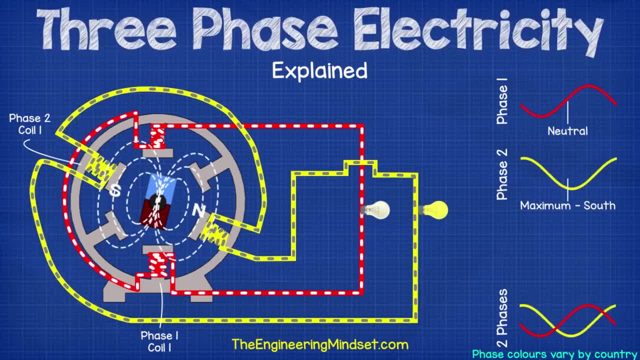 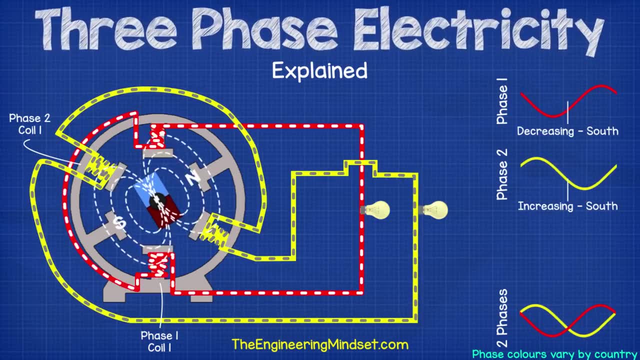 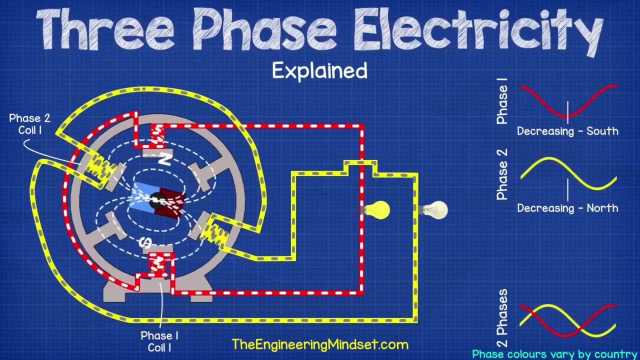 We can do this by placing the coils a 120 degrees rotation from the first set of coils and then connect this up to another lamp. This rotation means that the coils will experience the changing intensity of the magnetic field at different points in time. The first coil reaches its maximum current and brightness and as it decreases, the second 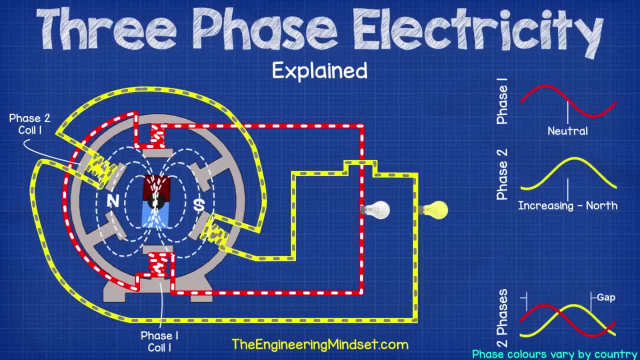 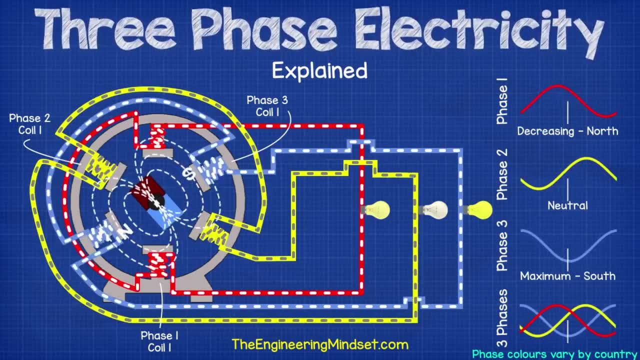 coil will begin to increase. This has improved the lighting, But there's still a lot of light. There's still a gap which will cause a flicker. So we can add in a third set of coils or a third phase, and this will mean that one. 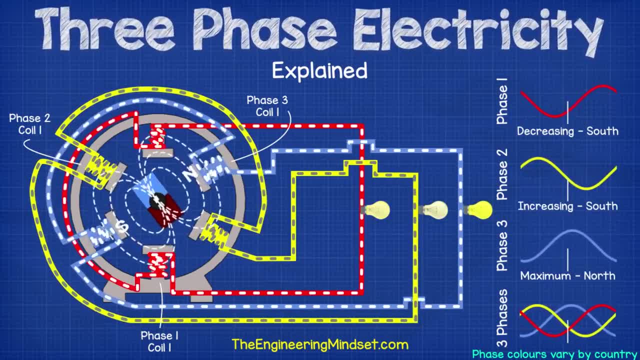 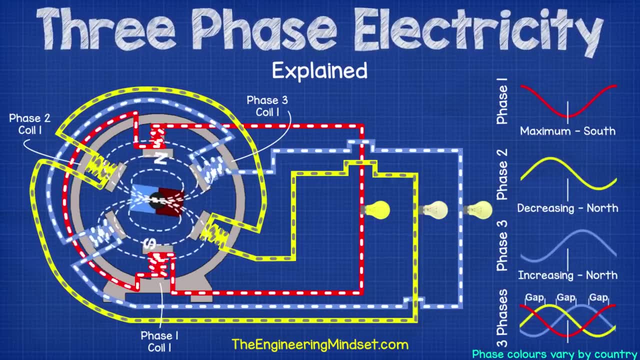 of the lamps are almost always at its maximum brightness, so the lighting is nearly constant. There are still some small gaps between the phases, and you could keep adding more and more phases to fill these gaps, but this will become more and more expensive to keep running. 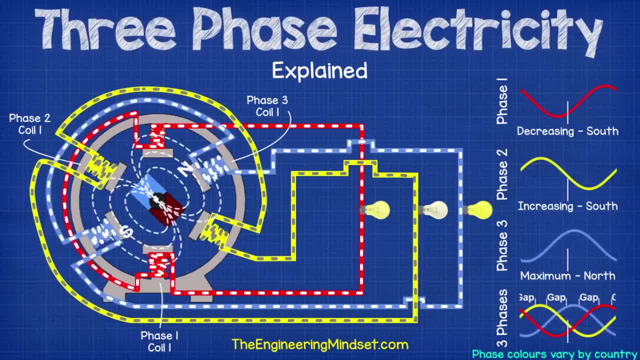 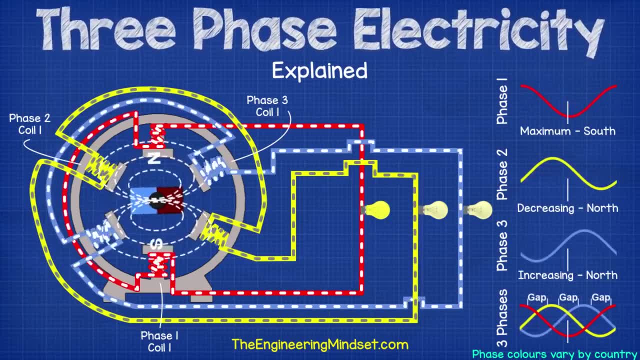 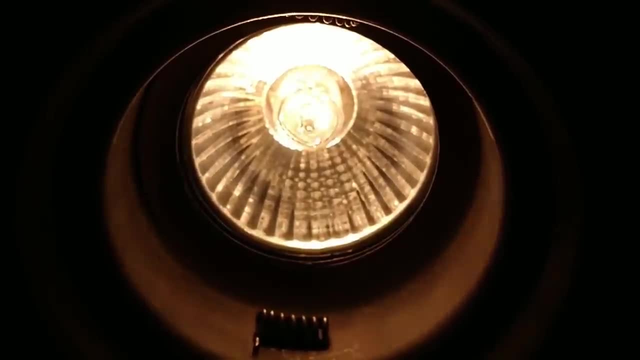 all these cables. So free phase became widely accepted as it's a good compromise between power provided and cost to build. Now, in the real world, you're not going to use three different lamps on different phases to create lighting. The lamps in your homes are all on single phase, but they are flickering, it's just.